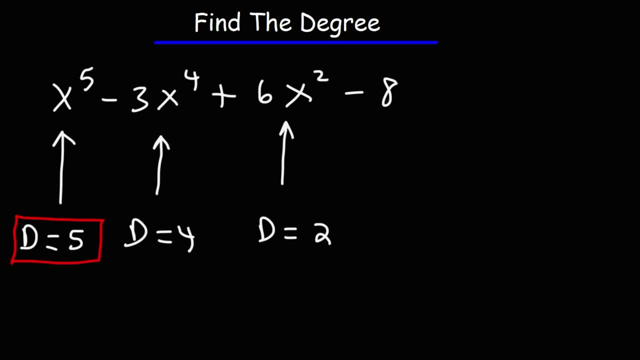 is 5.. That is our answer. So that's how you could find the degree of the polynomial. All you need to do is find the monomial with the highest degree, And that's going to be your answer. Now, for the sake of practice, let's go ahead and work. 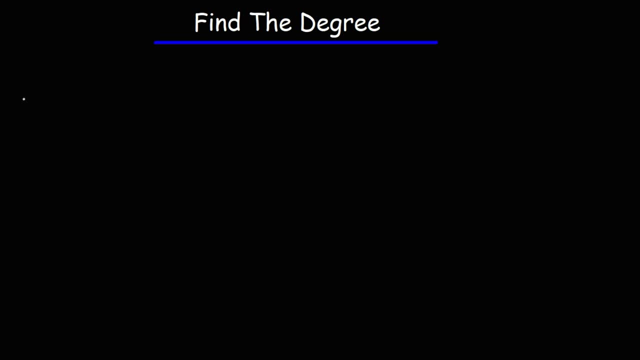 on some more examples. So try these. Let's say we have 2x to the fifth power, minus 6x cubed, plus 8x to the ninth power. And then for the next one, let's say it's going to be 3x to the fourth power. 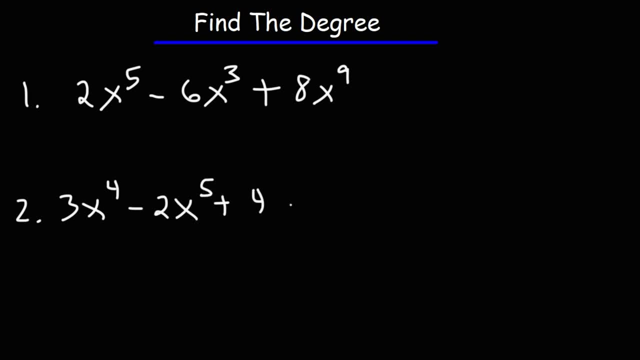 Minus 2x to the fifth power. So feel free to pause the video and try these example problems. So, looking at the first one: Minus, Minus, Plus, Minus, So this polynomial, we could say it's degree 8.. 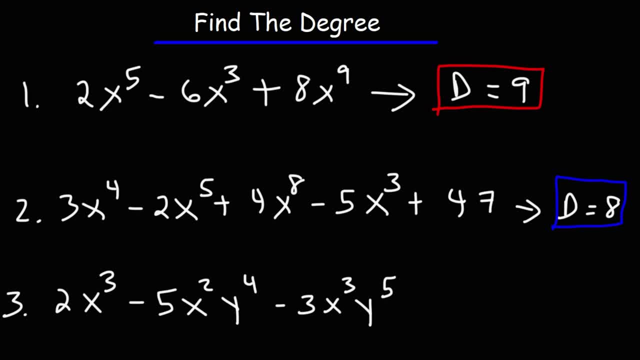 Now what about the last one? What do we do if we have a polynomial with multiple variables? In this case, you need to add the exponents. So let's do this one step at a time. The first term has a degree of 3.. 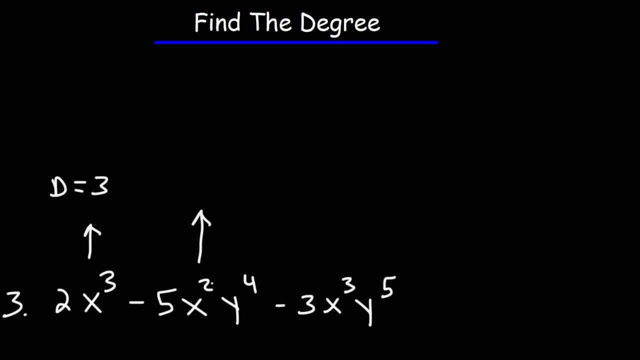 The second term. we have an x squared and a y to the 4th and we need to add the exponents. 2 plus 4 is 6, so the second polynomial has a degree of 6.. For the last one, it's 3 plus 5, which is 8.. 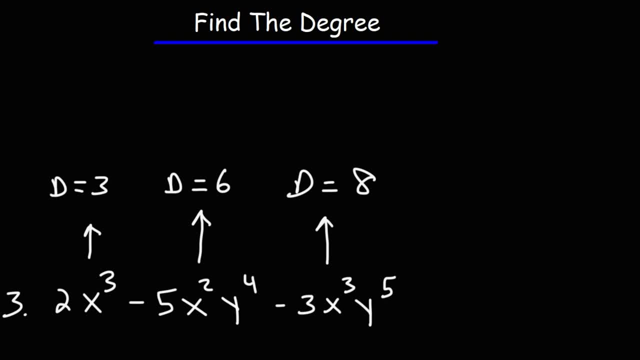 And so that's the highest degree. So our final answer is going to be degree 8.. So that's the degree for this particular polynomial. Now, let's do this one step at a time. Now let's try some other examples. 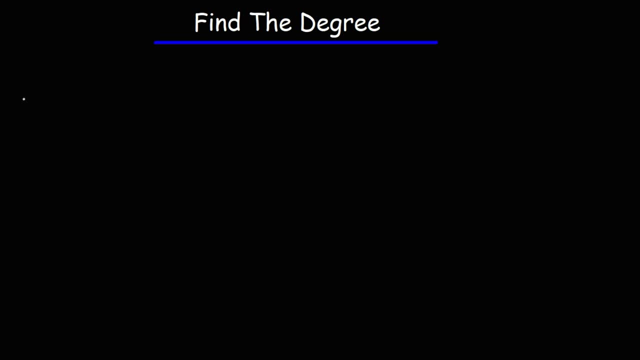 on some more examples. So try these. Let's say we have 2x to the fifth power, minus 6x cubed, plus 8x to the ninth power. And then for the next one, let's say it's going to be 3x to the fourth power. 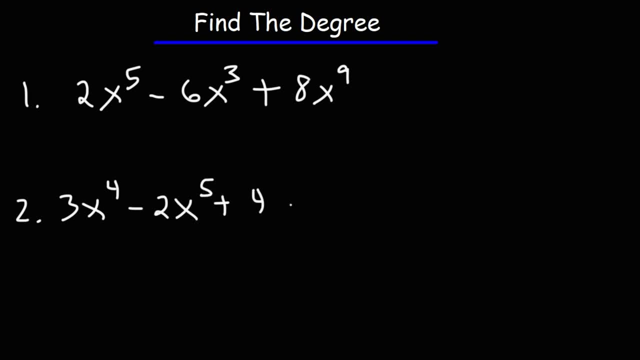 Minus 2x to the fifth power. So feel free to pause the video and try these example problems. So, looking at the first one: Minus 2x to the fifth power. Minus 2x to the fifth power. Minus 2x to the fifth power. 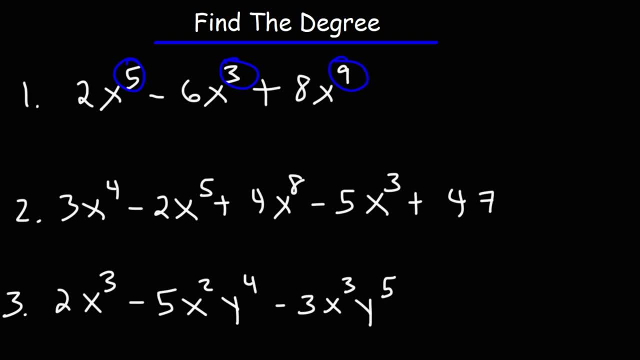 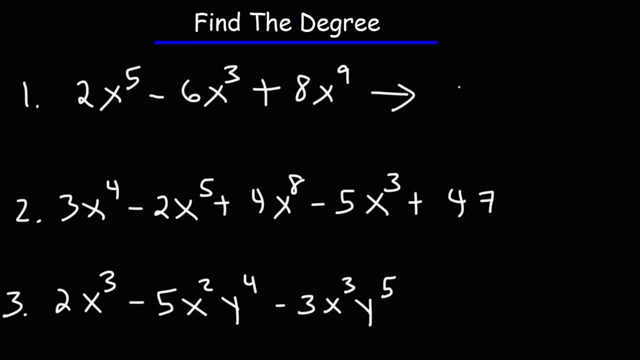 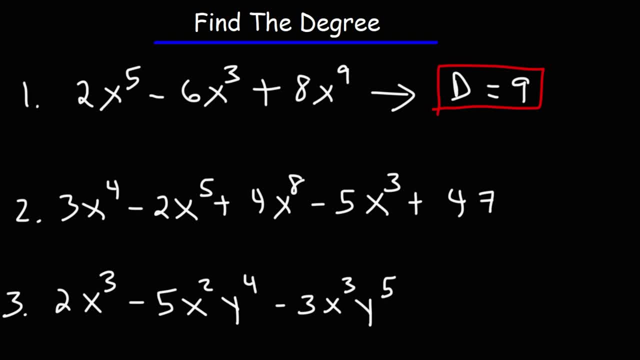 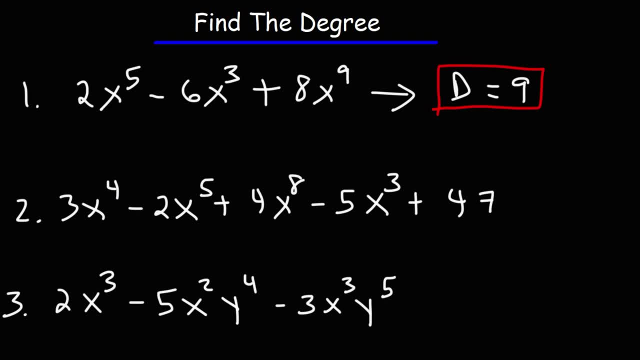 So 8 is the highest one. So this polynomial, we could say it's degree 8.. Now, what about the last one? What do we do if we have a polynomial with multiple variables? In this case, you need to add the exponents. 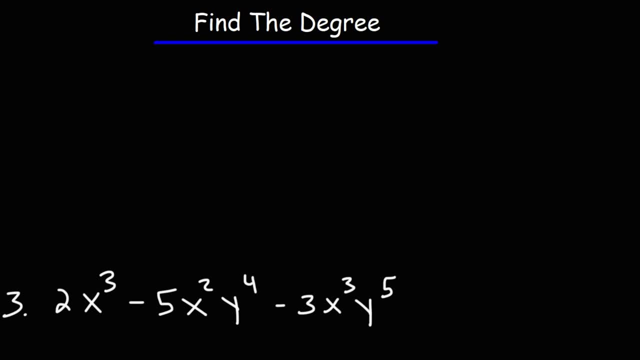 So let's do this one step at a time. The first term has a degree of 3.. The second term: we have an x squared and a y. to the 4th We need to add the exponents. 2 plus 4 is 6, so the second polynomial has a degree of 6.. 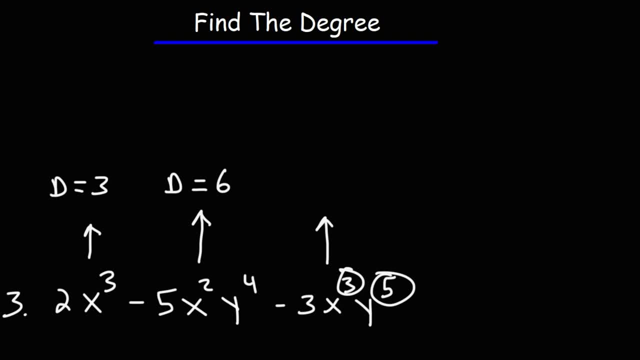 For the last one, it's 3 plus 5, which is 8.. And so that's the highest degree. So our final answer is going to be degree 8.. So that's the degree for this particular polynomial. Now let's try some other examples. 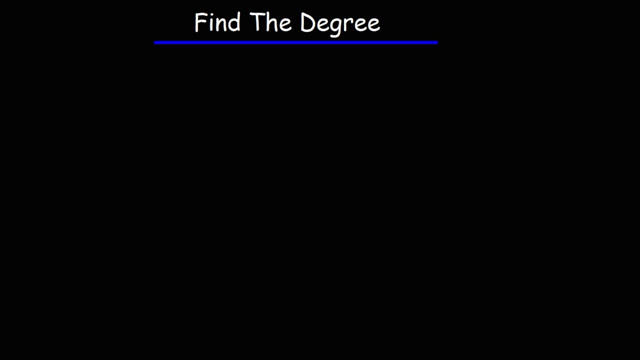 Examples that are slightly harder than the previous ones. So go ahead and try this. Let's say we have 4x to the 13, minus 3x to the 8th, y to the 9th, and then minus 4x to the 5th, y to the 11th. 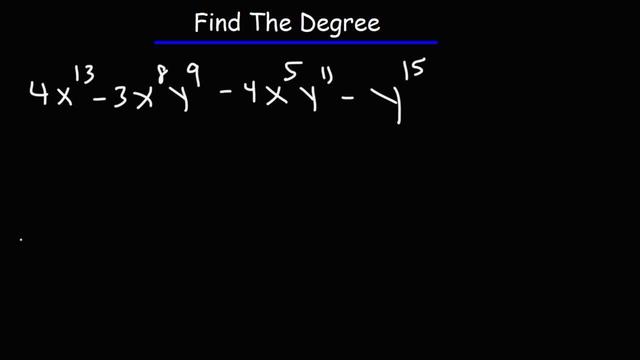 minus y to the 15th. and try this one as well: 3x squared y cubed z to the 4th, minus 5x cubed y squared z to the 5th. So go ahead and try those examples. 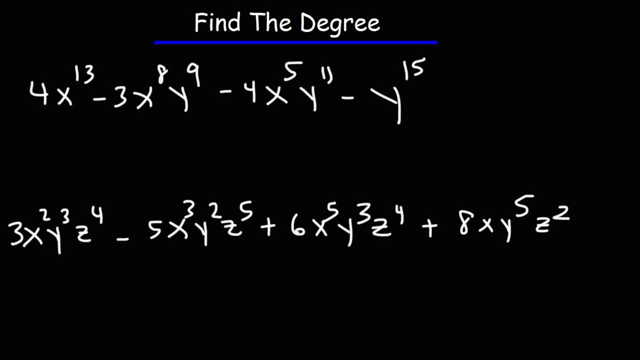 Let's find the degree of each monomial and then we'll identify the degree for the polynomial. So the first term has a degree of 13.. For the second one, if we add 8 and 9, that's going to give us 17.. 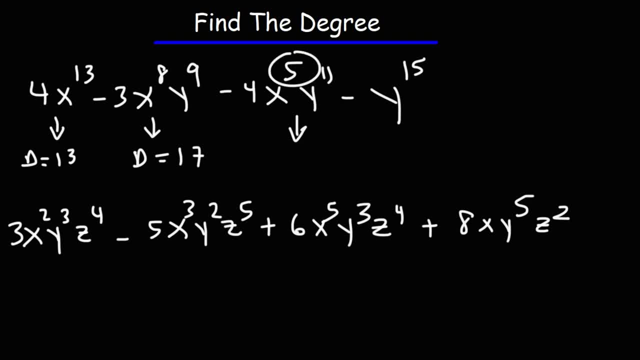 For the third term: 5 plus 11,, that's 16.. And the last one: we can see that it's going to be 15.. So the highest degree is 17,, and that is the degree for this entire polynomial. 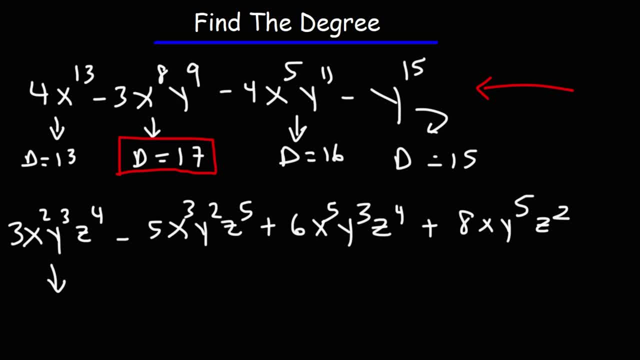 Now for the next example. we have a polynomial, not with two variables, but with three different variables: x, y and z. So let's find the degree of each monomial: 2 plus 3 plus 4, that's going to be 9.. 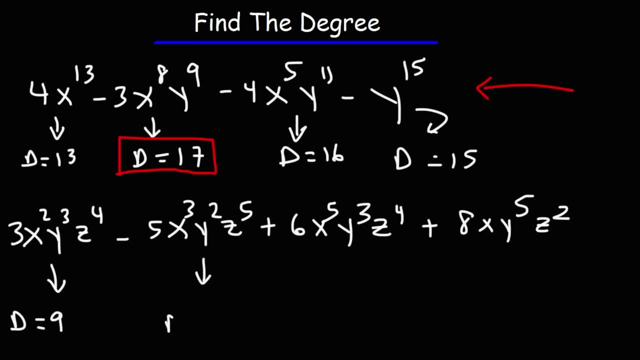 3 plus 2 plus 5, that's going to be 9.. 3 plus 2 plus 5, that's going to be 9.. That's going to give us 10.. And then 5 plus 3 plus 4.. 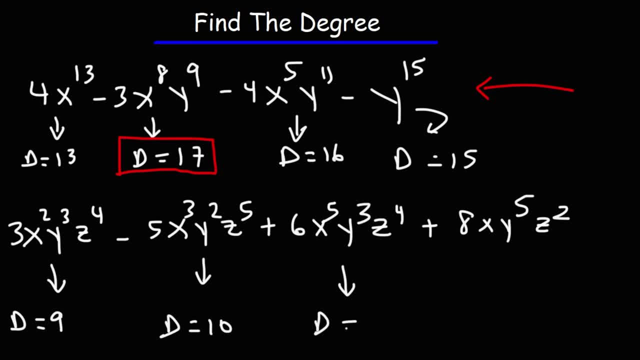 5 plus 3 is 8.. 8 plus 4 is 12.. So here we have an invisible: 1. Plus 5, that's 6. Plus 2 is 8.. So the highest degree is 12.. 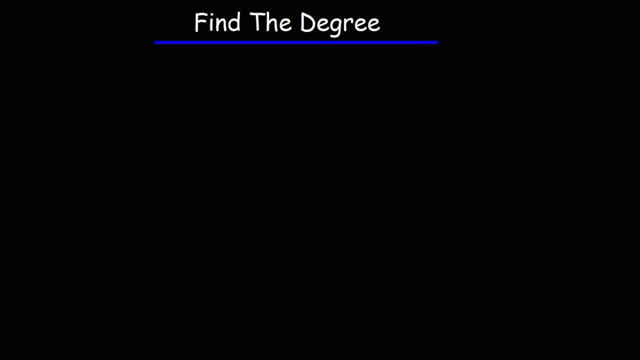 Examples that are slightly harder than the previous ones. So go ahead and try this. Let's say we have 4x to the 13th, minus 3x to the 8th, y to the 9th, and then minus 4x to the 5th, y to the 11th, minus y to the 15th. 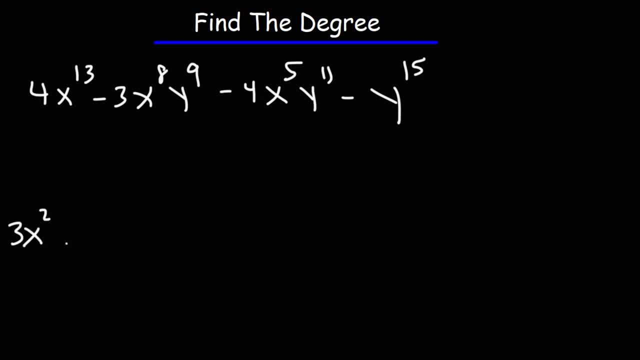 And try this one as well: 3x squared y cubed z to the 4th, Minus 5x cubed y squared z to the 5th. So go ahead and try those examples. Let's find the degree of each monomial. 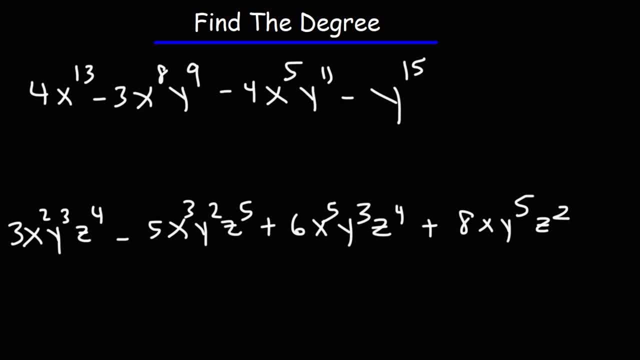 Let's find the degree of each monomial And then we'll identify the degree for the polynomial. So the first term has a degree of 13.. For the second one, if we add 8 and 9, that's going to give us 17.. 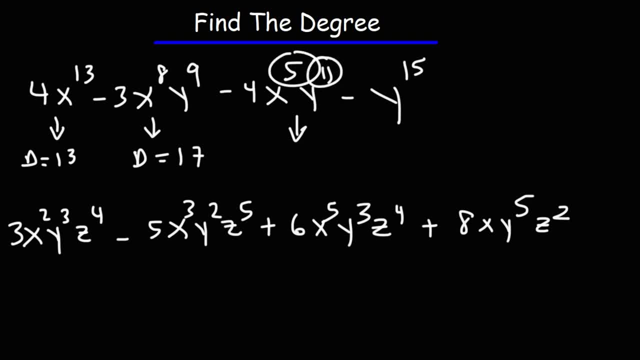 For the third term: 5 plus 11,, that's 16.. And the last one, we can see that it's going to be 15.. So the highest degree is 17. And that is the degree for this, And that is the degree for this entire polynomial. 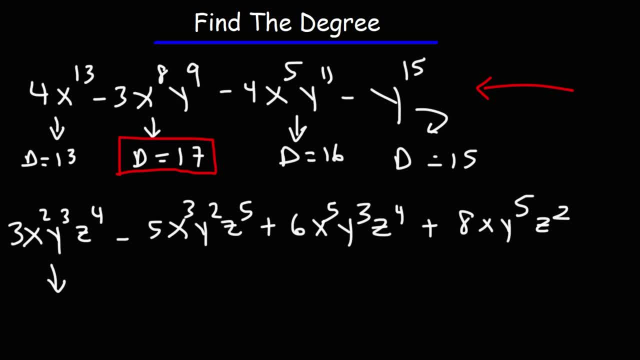 Now for the next example. we have a polynomial, not with two variables, but with three different variables: x, y and z. So let's find the degree of each monomial: 2 plus 3 plus 4, that's going to be 9.. 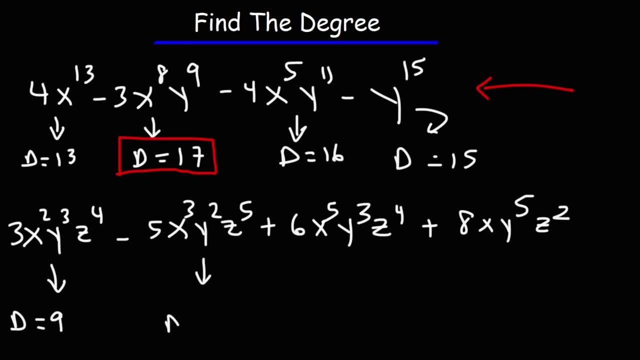 3 plus 2 plus 5, that's going to give us 10.. And then 5 plus 3 plus 4.. 5 plus 3 is 8.. 8 plus 4 is 12.. So here we have an invisible 1.. 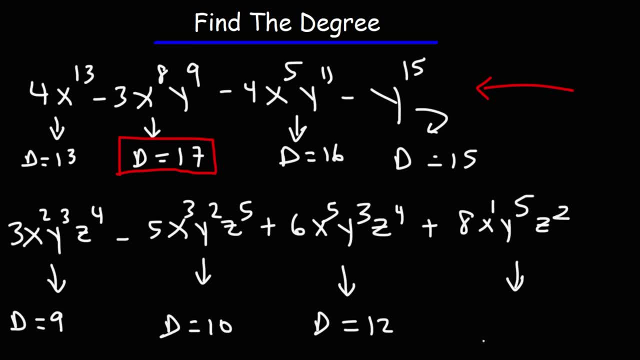 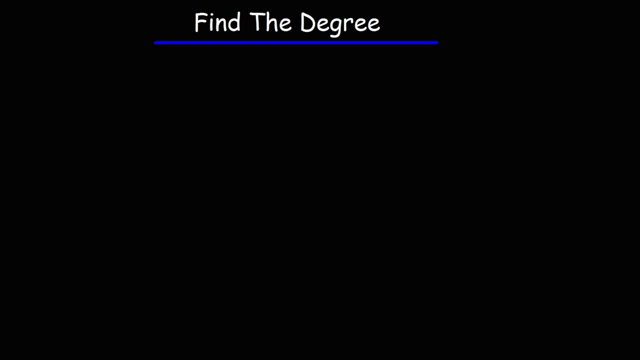 Plus 5,, that's 6.. Plus 2 is 8.. So the highest degree is 12.. So we can say that this polynomial has a degree of 12.. Now let's try a different example. Sometimes you may be given the polynomial in factored form. 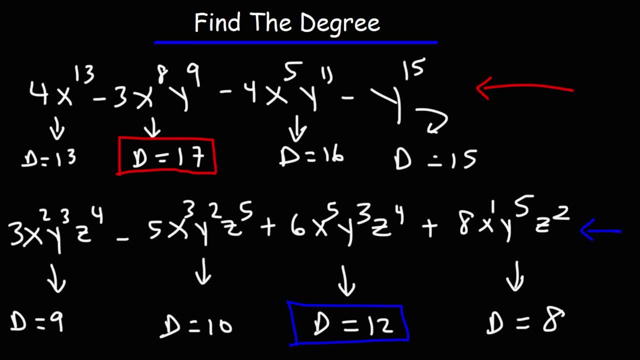 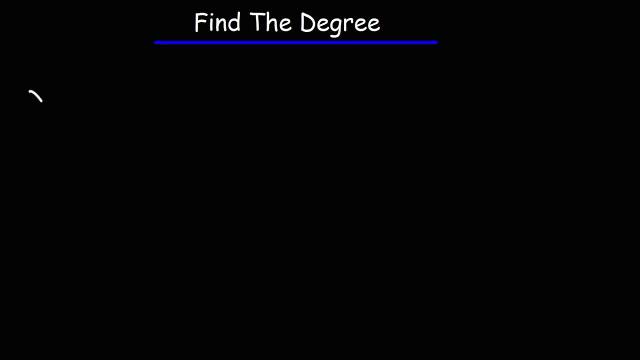 So we can say that this polynomial has a degree of 12.. Now let's try a different example. Sometimes you may be given the polynomial in factored form. So let's say you get a question that looks like this: 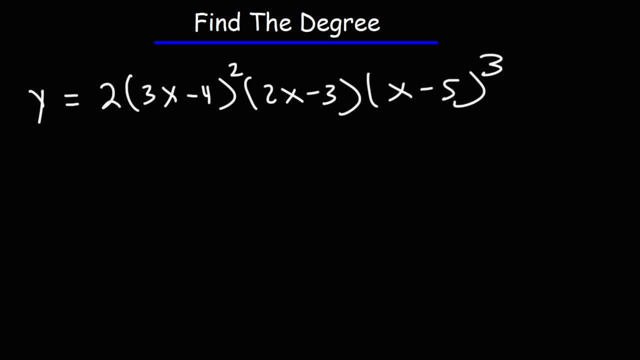 What is the degree of the polynomial? You could find the answer by finding the degree of the highest term. So here we have a 3x which is x to the first power and it's raised to the second power. So if you were to FOIL 3x minus 4 times 3x minus 4, the term with the highest degree will be 9x squared. 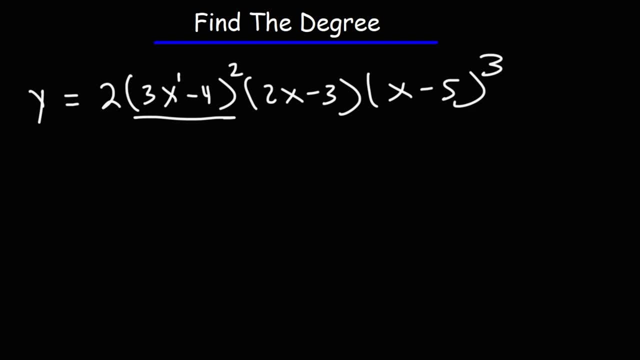 But we don't need to worry about the 9. We just need to focus on the x squared part. So the highest term is going to be x to the second power For this one. this is x to the first power raised to the 1.. 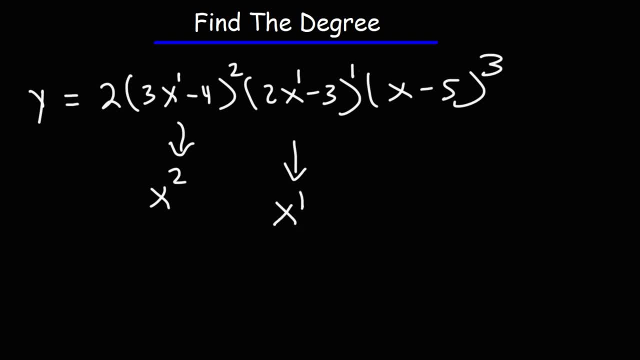 1 times 1 is 1.. So the highest term will be x to the first power For this one. this is x to the first. raised to the third power, 1 times 3 is 3.. So the highest term here will be x cubed. 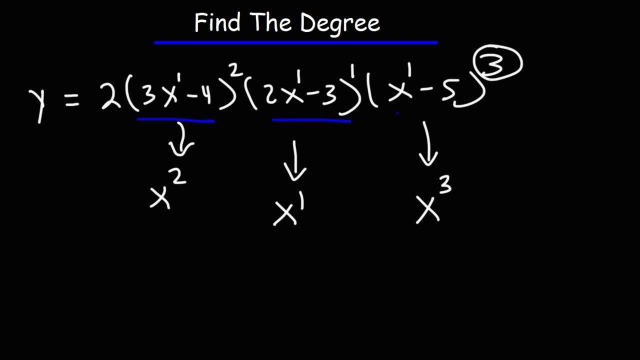 Now these values here? they're not added to each other, They're multiplied. So we need to multiply Those three- x squared times x times x cubed, To get the answer. we need to add the exponents. Anytime you multiply the same variable, you need to add the exponents. 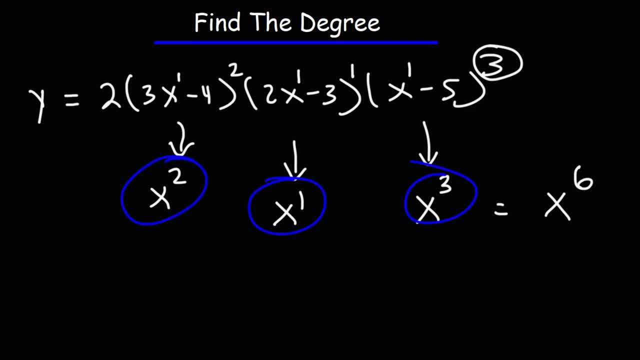 So this is going to be 6.. So this polynomial has a degree of 6.. And that's how you can find the answer if you're given the polynomial in factored form. Now let's try another example. So let's say we have: y is equal to 3 times x minus 2, raised to the third power. 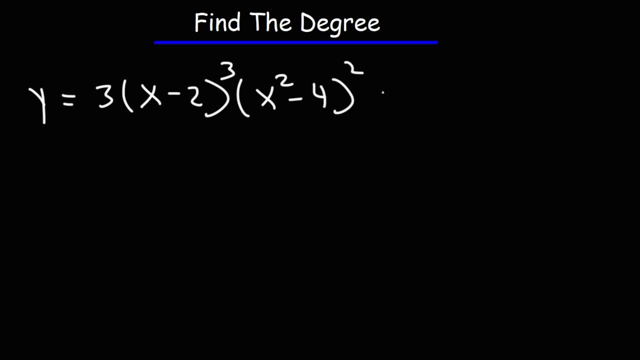 And then x squared minus 4, raised to the second power, And then x cubed minus 5, raised to the fourth power. Go ahead and find the degree of this polynomial. So this is x to the first, raised to the third power. 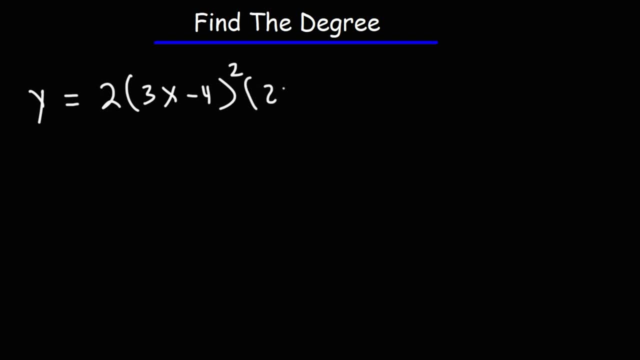 So let's say you get a question that looks like this: What is the degree of the polynomial? You could find the answer by finding the degree of the highest term. So here we have a 3x, which is x to the first power. 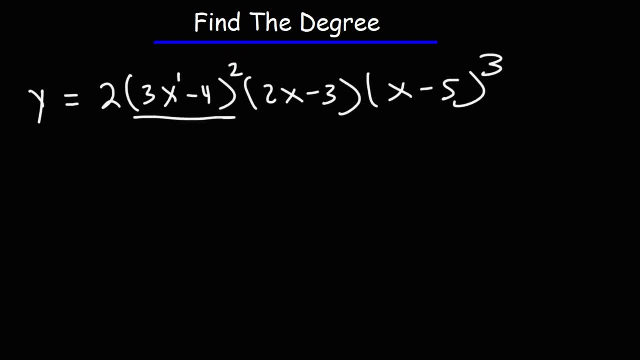 and it's raised to the second power. So if you were to FOIL 3x minus 4 times 3x minus 4, the term with the highest degree will be 9x squared, But we don't need to worry about the 9.. 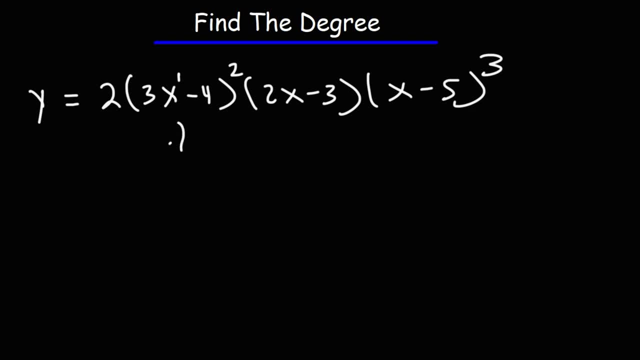 We just need to focus on the x squared part, So the highest term is going to be x to the second power. For this one, this is x to the first power. raised to the 1.. 1 times 1 is 1.. 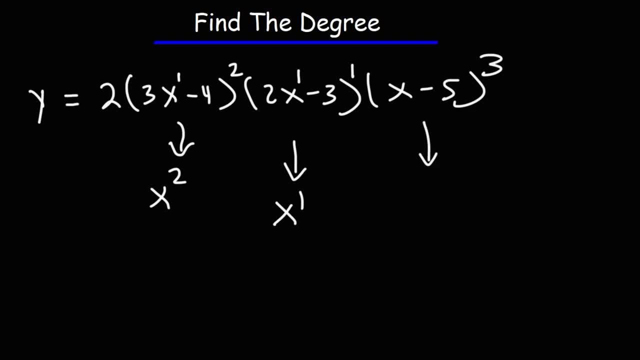 So the highest term will be x to the first power. For this one, this is x to the first. raised to the third power, 1 times 3 is 3.. So the highest term here will be x. cubed Now, these values here, they're not added to each other. 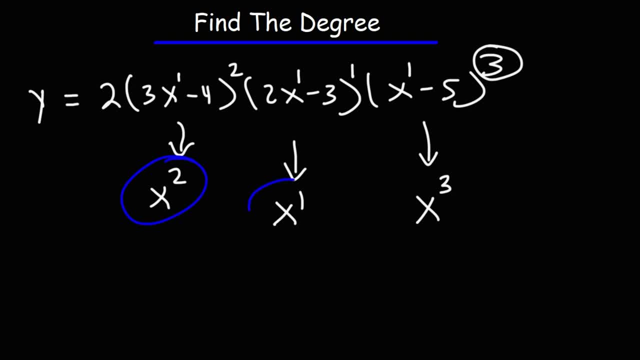 They're multiplied. So we need to multiply those three- x squared, times x times x cubed- To get the answer. we need to add the exponents. Anytime you multiply the same variable, you need to add the exponents. So this is going to be 6.. 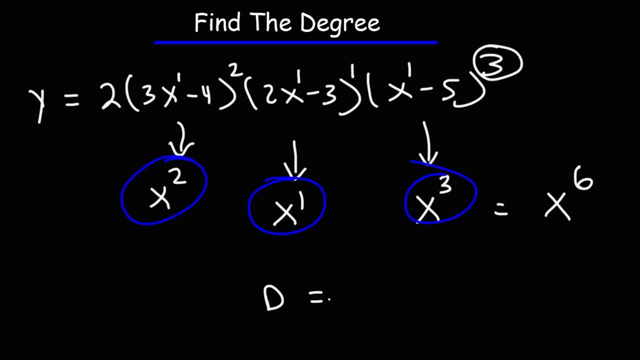 So this polynomial has a degree of 6. And that's how you can find the answer if you're given the polynomial in factored form. Now let's try. Let's try another example. So let's say we have: y is equal to 3 times x minus 2, raised to the third power. 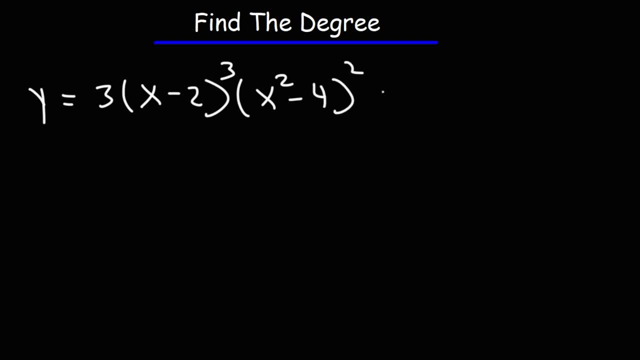 And then x squared minus 4, raised to the second power, And then x, cubed minus 5, raised to the fourth power. Go ahead and find the degree of this polynomial. So this is x. This is the first raised to the third power.